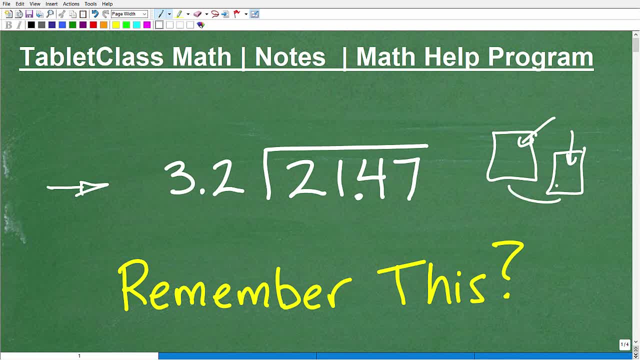 I have my computer, I have all this wonderful technology, So I don't really need to remember how to do this. Well, you couldn't be more incorrect with that perception. right, You need to be strong in arithmetic. Now just think about it If you, you know, one day you lost your cell phone or didn't have your calculator, or whatever the case is, and you had to do some basic. you know calculations, you know maybe, trying to figure out a money situation, or something like that. 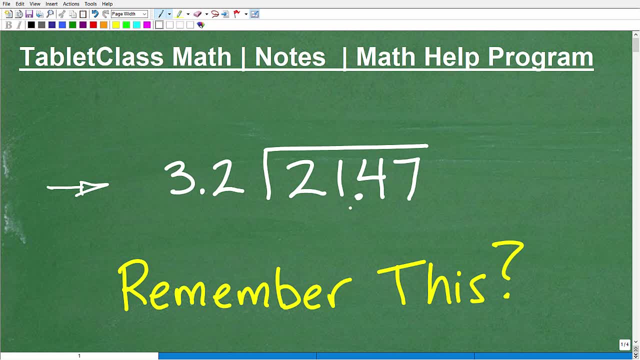 You still need to know how to do arithmetic Now. I know it's not a common skill that we practice, but let's try to practice this now. Now just a quick story before I get into this problem. Way back in a former life I served some time in the military. Now I was a Navy surface warfare officer. Okay, that meant, you know, I drove Navy ships. and here I'm a little Navy ship here like. so Now, the little thing I'm telling you here. it goes to what 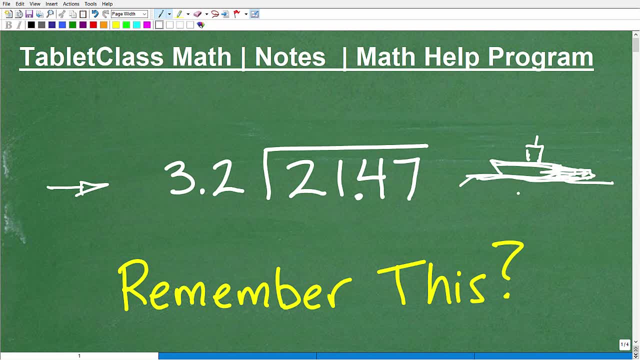 the main point I'm talking about Now around the year 2000,. there was something called Y2K. I don't know if any of you have heard about that. It's kind of in the history books right now. But everybody was very concerned that when we went from 1999 to the year 2000, that all the computers were going to blow up and everything was going to go, you know, very, very bad. That was a real legitimate concern. 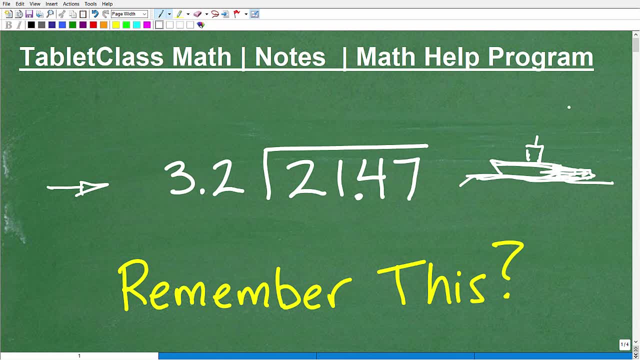 Anyways, my point is this: on naval ships, the way we find our position is using something called GPS, right? So, just like you know on your cell phone, when you go and plug in your Google Maps, we know our actual location, etc. By GPS. Well, at Y2K, that time there was a big concern, that you know. we didn't really know how the satellites and everything else were going to be This particular time, and when I was finished finishing up my naval career, I was actually a navigator. 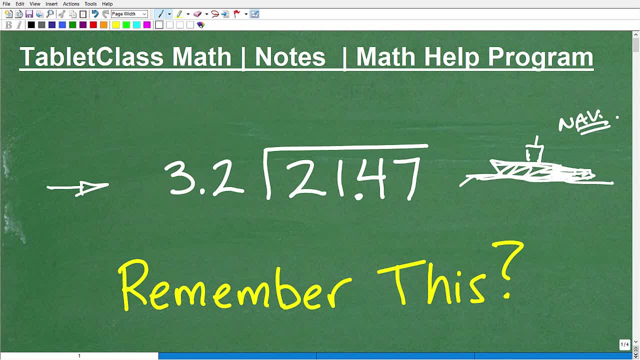 Okay, which was awesome, I was able to use my mathematics skills, but I navigated a gigantic Navy warship. Okay, a lot of responsibility, But what I'm getting at is this: We had to really really ensure that we had our celestial navigation skills down, So, basically, we could find our position by the stars, And it wasn't just us, It was all other folks that were, you know, concerned with maritime stuff or whether it be aviation. 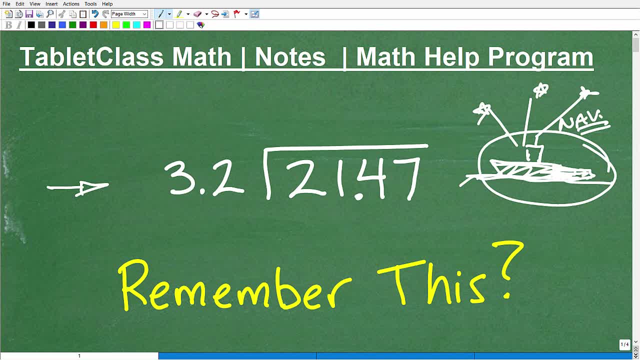 And this is kind of like old school skills. This would be like equivalent to knowing arithmetic. When your calculator breaks down, you still had to know the old way of doing things by hand. Okay, so you can't be overly dependent on technology, because you just never know when you may not have that lovely technology that we enjoy so much available. Okay, so arithmetic is very, very important And 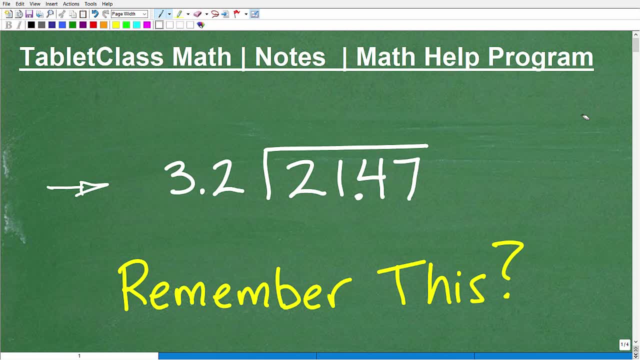 you'll got to know it. So if you're like I don't know if I remember how to divide decimals, Well, we're going to do this quick problem And this is just a quick refresher. It's not going to be a complete, full lesson on this, So we're going to do this in just one second. But first let me quickly introduce myself. My name is John. I'm the founder of tablet class math. I'm also a middle and high school math teacher And over several years I've constructed what I like to believe is one of the best online math help programs there is. Of course, I'll let you be the judge of that. If you're interested, you can check out my math help program by. 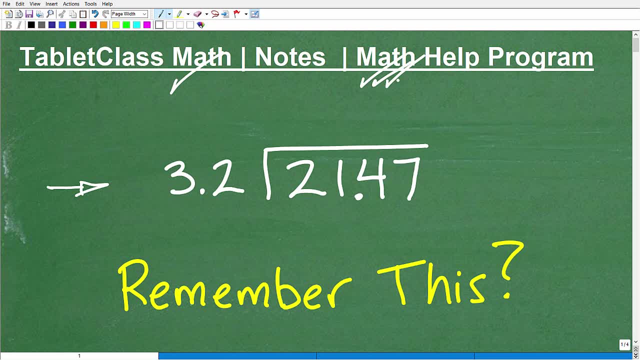 following the link in the description of this video. But basically I have 100 plus different math courses ranging from pre algebra, algebra and geometry, algebra two- I'm going to be launching pre calculus here shortly. But I also have many, many courses in the area of test preparation. So if you're studying for the GED, SAT, ACT now, GRE, GMAT, ASVAB, ACUPLACER, ALEKS exam, CLEP exam, maybe a teacher certification exam, maybe a nursing school entrance exam, all those 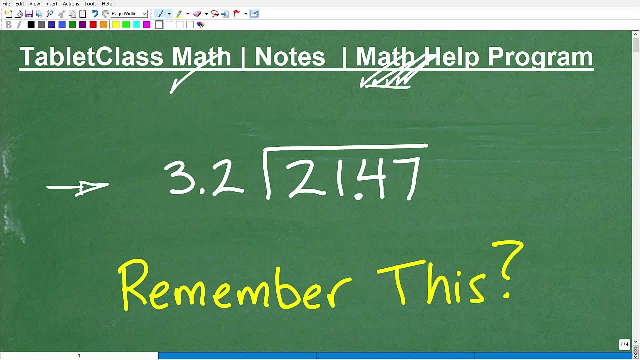 exams and many others have a lot of math on them. If you don't do well on the math section, you don't do well on the exam. So let me help you prepare. Just go to my site and check out my full course catalog. If I don't have the test you're looking for, drop me a line and I'll help you out the best I can. I also do a lot with homeschoolers, So if you homeschool, I have a great homeschool learning system- Definitely want to check that out And then obviously help those of you that are just struggling in your current math courses. Now, if you are truly serious about wanting to improve and learn mathematics, then you got to. 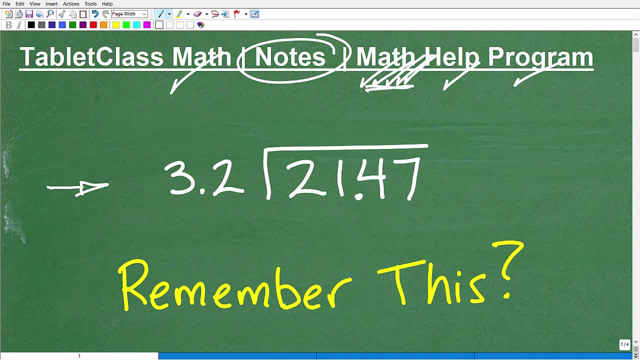 be serious about note-taking. Over decades of teaching math, this is kind of like my golden rule. When I see students every day working hard, taking excellent notes, they almost always end up with these kind of grades. And then the opposite is true- Those students who are like me. way back in the good old 1980s: what was I doing? I was taking notes, but they had nothing to do with math. During math class I was writing to my friends saying, hey, what are we doing this weekend? And then they would write back and et cetera, et cetera. We were very proud of ourselves. because we were doing great math, And then we would write back and et cetera, et cetera. We were very proud of ourselves because we were doing great math, And then we would write back and et cetera, et cetera. We were very proud of ourselves. 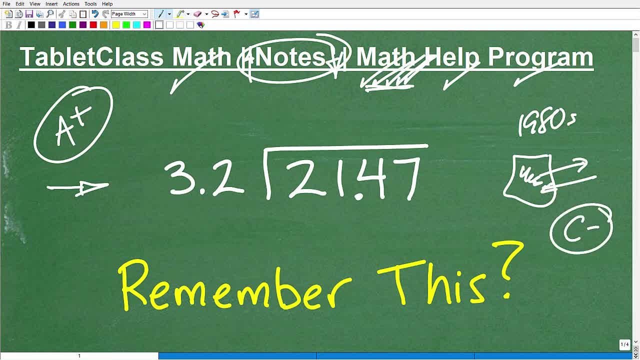 but then we would end up with grades like this. So there's no shortcuts. When you're in math class or any class for that, you got to buckle down and say to yourself: okay, I got to be focusing on note-taking, And that's the key word: focus. Okay, there is no shortcuts. You can't get out of taking great math notes if you're serious about doing well in mathematics, But you can use my notes as you improve your notes. And my notes include pre-algebra, algebra one, geometry, algebra two and trigonometry. You can find the links to those notes in the description. 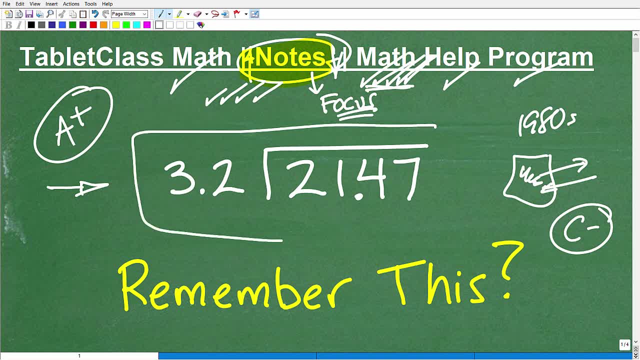 the description of this video. All right, let's get to this fun decimal division problem Now. obviously, I would like you to pause the video and try this on your own, without the aid of a calculator or technology, But you need to know something about basic division. Okay, so if you forget how to do some of the stuff that I'm going to go over and you might have learned this a little bit differently. Really, what I'm most interested in is like. however, you learned arithmetic, if you can get the right answer. 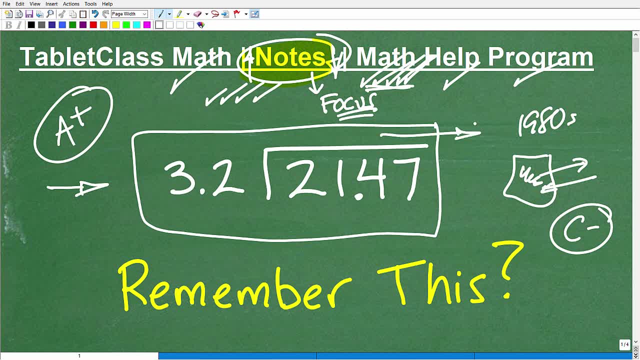 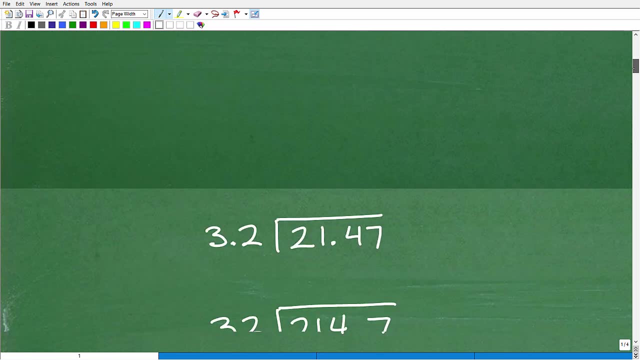 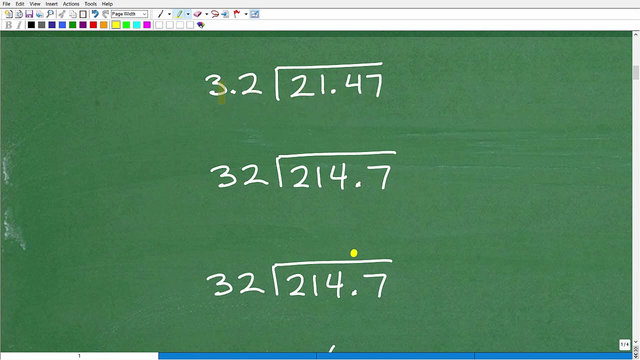 now, by the way, we can continue to go and, excuse me, create more, make our answer more accurate by adding more digits, But we'll do a few extra digits here And you'll see what I'm talking about in just one second. So let's get right to it And have some fun with dividing decimals- everyone's favorite topic. All right, So we have a 21.47. And we've got three 3.2,. we're gonna divide it into 21.47.. So what is the first thing we do? 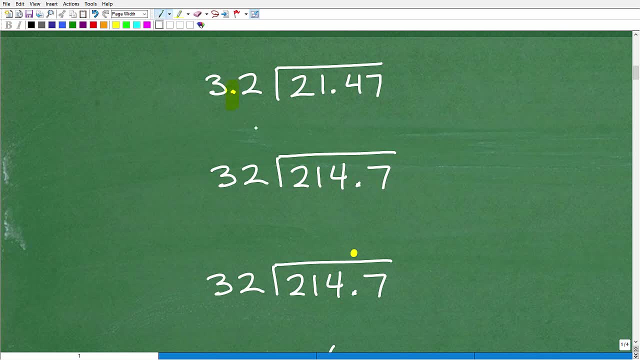 When we're dividing decimals. Well, we have a decimal point here. The first thing is that we got to deal with this And we got to move that decimal point over, like so, So it becomes a whole number. That is the first step you do, Okay, so this 3.2, we got to move the decimal point over once a spot, So it becomes a whole number. Now, because I moved it over one, these decimal points are kind of connected at the hip, if you will. they're kind of you can. 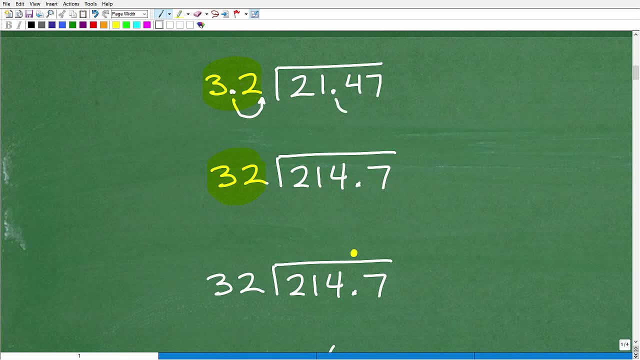 move them in tandem. So it's like, okay, move this over one, we're going to move this guy over one as well. So our problem becomes 32.. Okay, this is now 32.. And this is 214.7.. All right, now we're going to basically use the same division algorithm, the same steps as if we were doing this problem: 32 divided by 2147.. So here there's no decimals here. 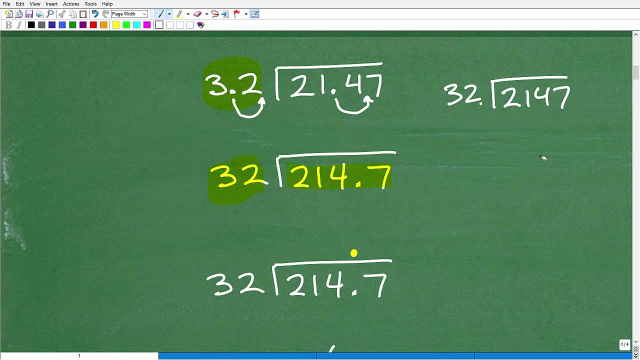 Obviously, there's a decimal right here, there's a point zero, But you got to be able to do a problem like this. Okay, if you can't do this problem, then you're not going to be able to do this. do this problem. But the steps that we take to the algorithm that we take to do this division problem is what we're going to be doing here. So when we're dividing decimals, it's really no different than doing this problem. All we're doing is moving the decimal point over. Now, what does that mean? Okay, when we move the decimal point over, we're going to be doing this. So when we're dividing decimals, it's really no different than doing this problem. All we're doing is moving the decimal point over. Now, what does that mean? Okay, when we move the decimal point over, we're going to be doing this. So when we're dividing decimals, it's really no different than doing this problem. All we're doing is moving the decimal point over. 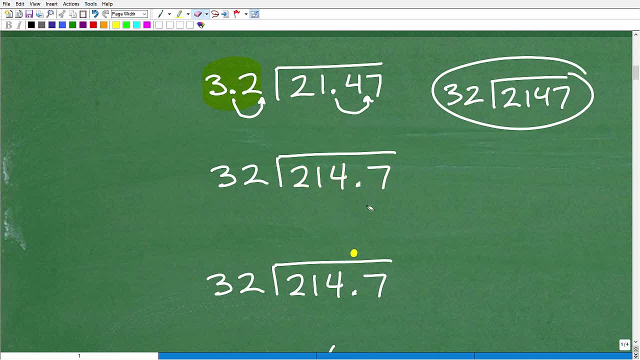 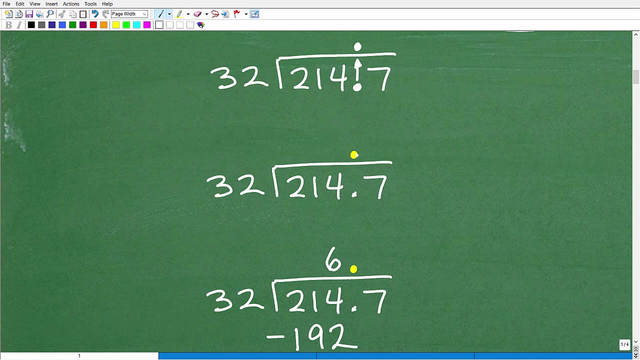 When I did that. okay, I'm kind of ready to start doing my division algorithm. Here's my decimal point. So my in my final answer, my decimal point is going to reside right there, after that four and before that seven. So that's what kind of have a kind of very prominent right here. Okay, so this is the setup. We don't have to guess where the decimal point is going to be. It's going to be right there. So let's go ahead and start. Okay with that. 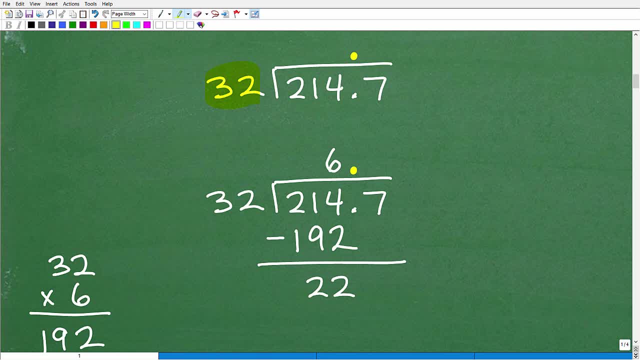 Basic division. So what does that look like? Well, 32.. I'm saying, okay, 32, I got to divide it into. can 32 divide into 21? No, they can't. But 32 could definitely go into 214.. So then this is where you, mentally, you have to start going like this: you have to say 32.. Can it go into it one? Well, obviously definitely can go into it twice, because that's 64. And then you just keep going up and up and up. You start testing numbers. just like you know, you learn back in elementary, primary. 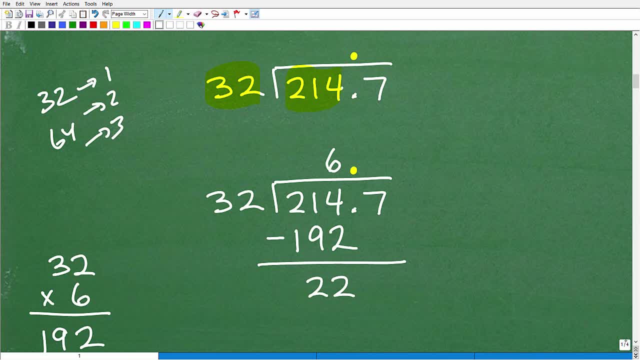 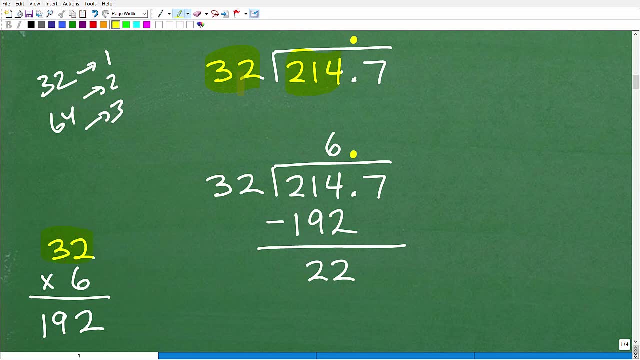 school and you figure out: oh, I can get 632s into 214.. All right, and you do this by kind of trial and error. So you got: 32 can go into 214 six times. All right. so 32 times six is 192. All right. So again, this is division that hopefully you've already learned. So we're saying, okay, 32 goes into 214 six times. So we go, six times 32 is that's 192.. So we're going to. 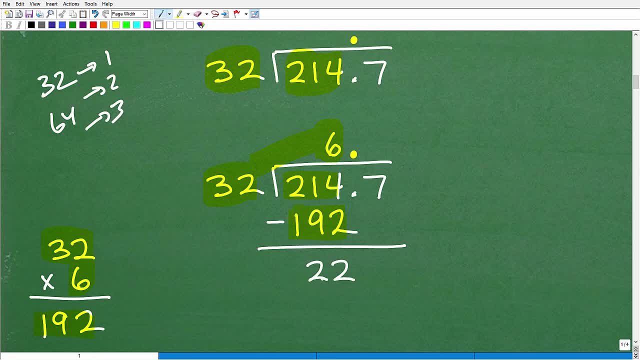 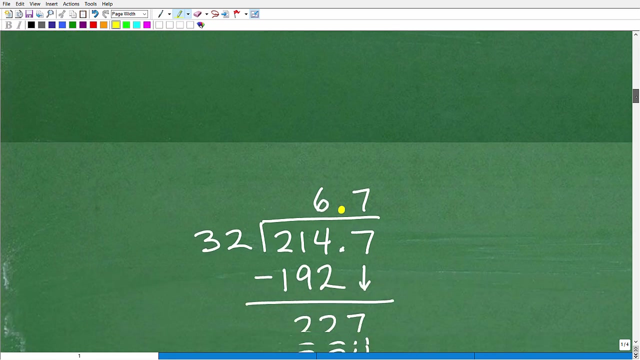 subtract that 192 from that 214. And I end up with 22.. Okay, so this is kind of the first part of this problem now, after we move the decimal points. And so now we we ask ourselves: can 32 go into 22?? And the answer is no. So what do we do? Okay, well, what we do is the following: All right, let me go ahead and continue the problem here. All right, so 32 could not have gone into. 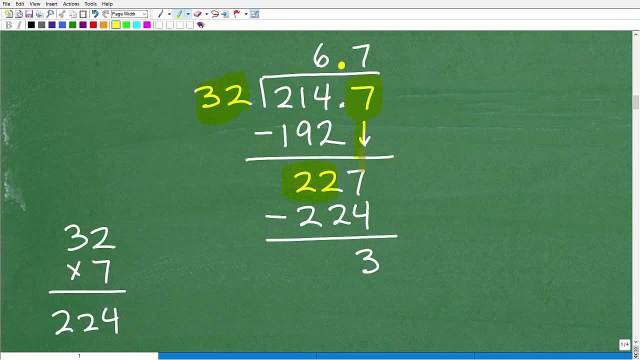 22.. But we got this lovely seven over here, So we're going to drop it down. All right, this is what we do in division, And now we're going to put it behind this 22,. this becomes 227.. So 32 definitely can go into 227. And we do the same thing in our brain. we know, okay, 32 times one, definitely times two, that can go into it. and you kind of keep going And you say: Oh, I can go up to seven. So 32 times seven is 224.. So 32 goes into 227, seven times. 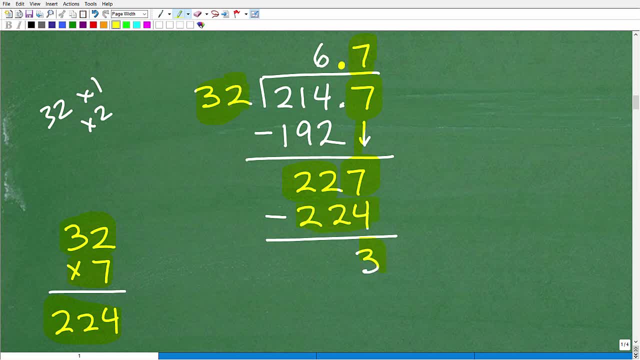 all right. so seven times 32, that's 224. And when we subtract we end up with three. Now this, this steps that I'm doing here. this is what we call the division algorithm. As I stated before, we did this problem, you got to know how to do basic division, Okay, so hopefully you know. if you don't remember that, then this is obviously going to be more confusing. All right, so here we are effectively kind of done. All right, So 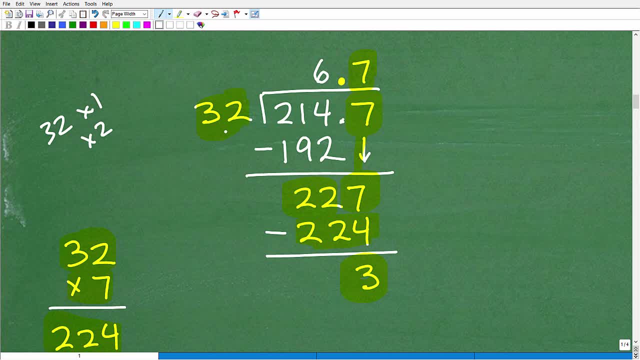 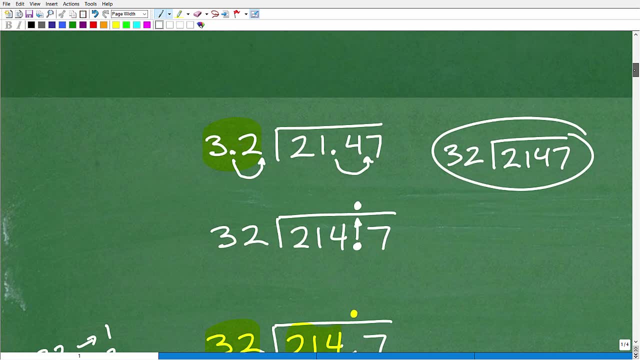 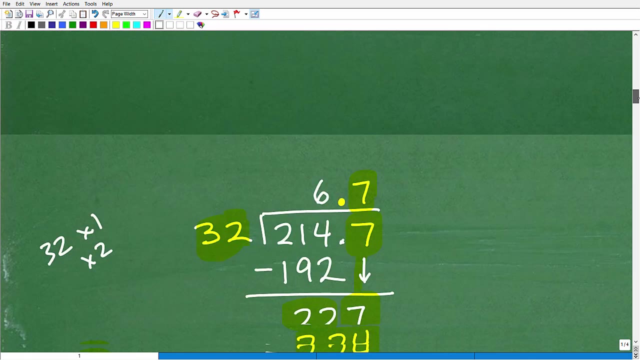 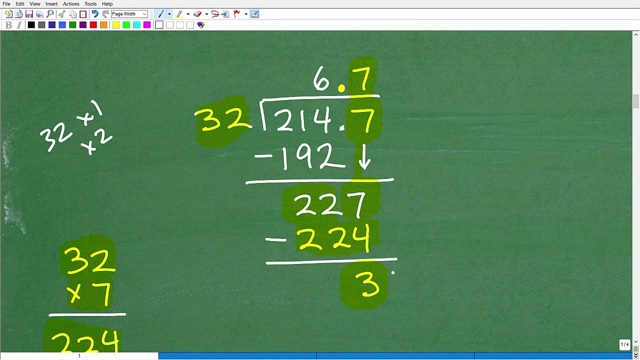 214.7 divided by 32.. All right, or the equivalent decimal answer here, or decimal version of the problem, which is 21.47 divided by 3.2.. Okay, what we have so far is 6.7.. Now some of you might say: well, okay, I know, 32 can't go into three, so we can stop. So this is a decent estimate. But let's say we wanted to keep going and get a more precise answer. 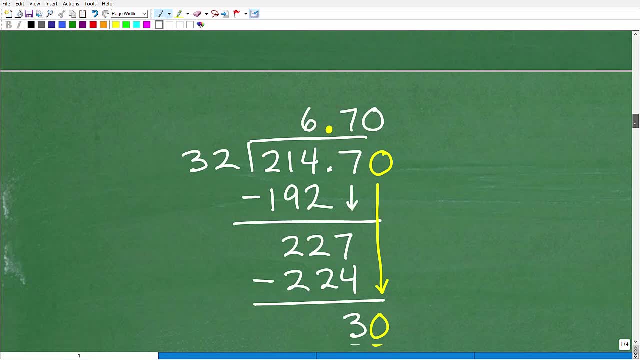 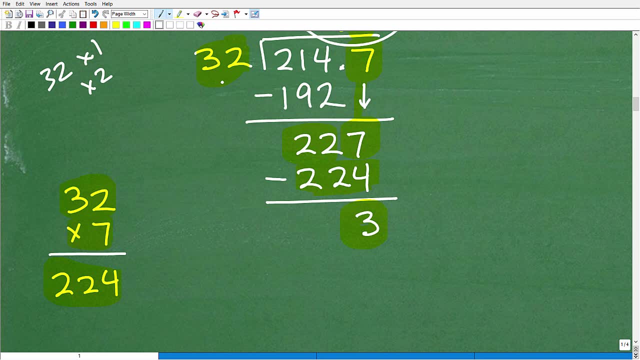 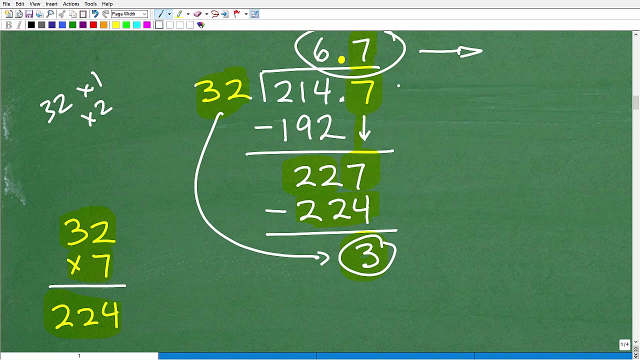 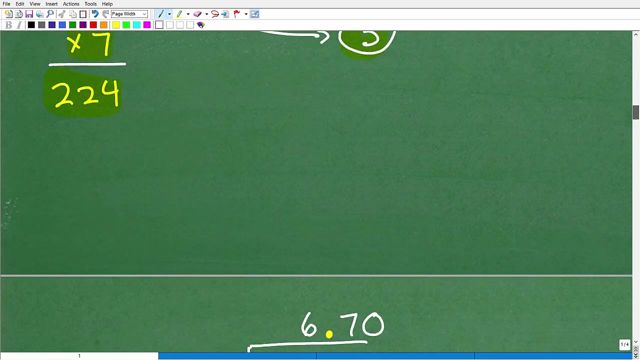 How can we do that? Well, this is what we're going to do. So we're like: okay, we know that 32, let's back up here real quick. So we know that 32 can't go into three. Okay, so we're kind of stuck. And then, here, seven was our last digit. But we're like, well, it would be nice if we could drop a digit down. Well, we can always drop a zero down. Okay, so that's exactly what we're going to do. Okay, so we're going to write a zero here. 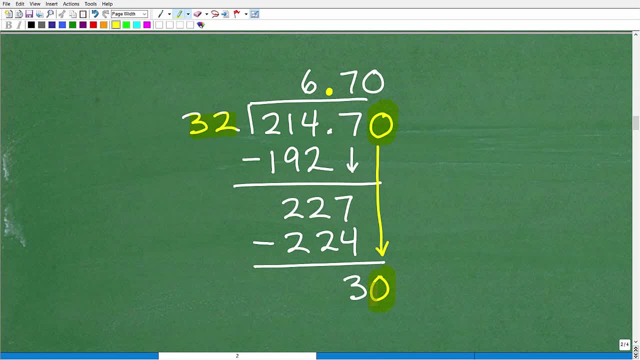 going to drop it down right here. Now I'm going to say, OK, can 32 now go into this number? 30? No, it cannot. So at this point we put a zero Right. That's important. This is part of our. 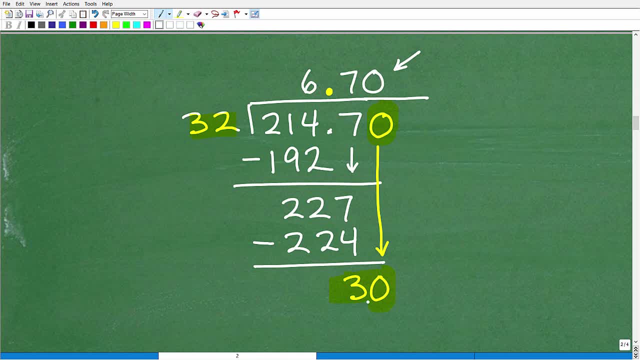 answer now. So 32 cannot go into zero, I mean 30,, 32 can't go into 30. So we put a zero as our answer. So we're like, OK, well, how can we continue to get an even more precise answer? 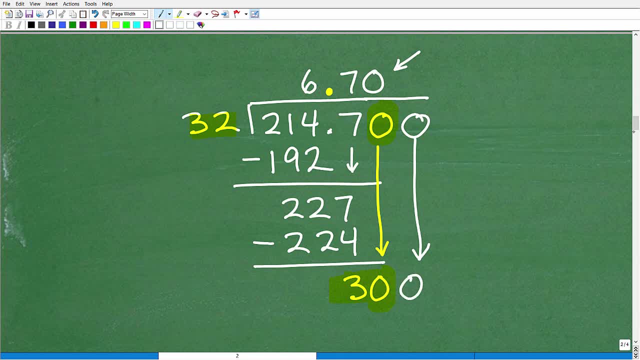 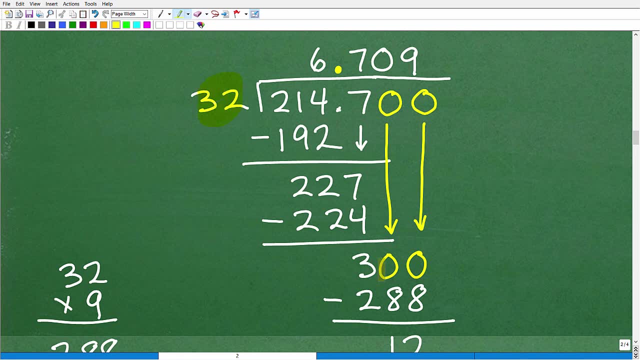 Well, you guessed it, We can even put another zero down here, And that's exactly what we're going to do. OK, we're going to drop another zero down. So finally, we got 32.. Couldn't go into 30, but it definitely goes into 300.. So 32 goes into 309 times. OK, so 32 times nine is 288.. 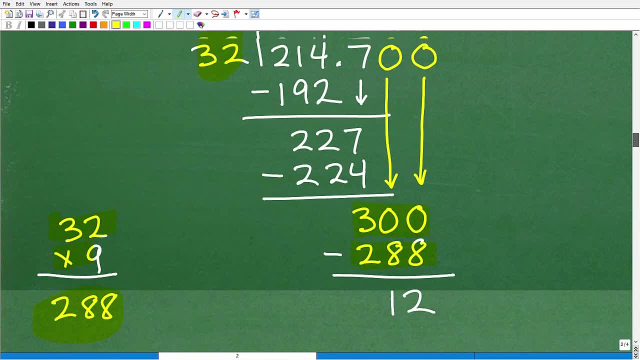 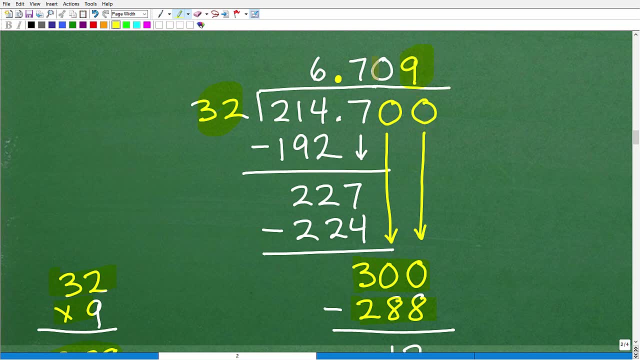 So we'll put our 288 right there. All right, 32 times nine- You can see the work right there, And I got to put the nine above that zero right there. OK, so nine times 32 is 288.. And I subtract. 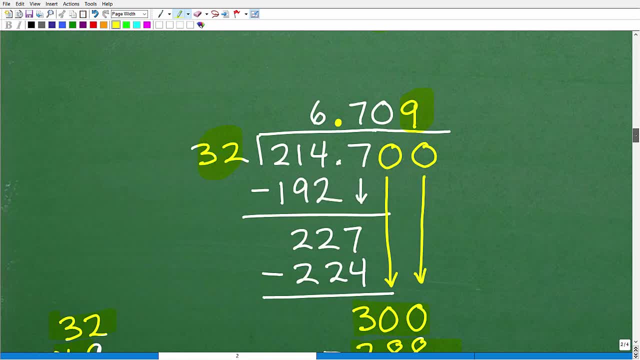 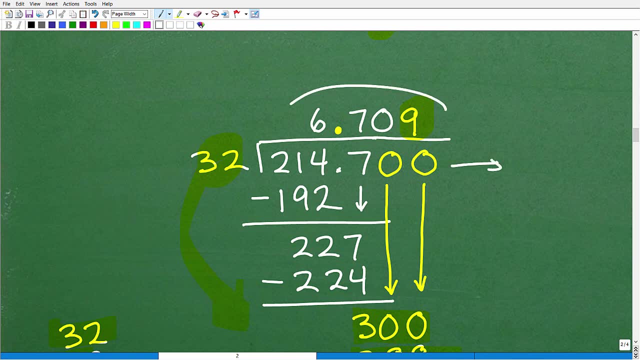 and I get 12.. Now, obviously 32, this 32 can't go into that 12. And we could just continue on the process, et cetera, et cetera. just refining our decimal answer. OK, do we get you know? 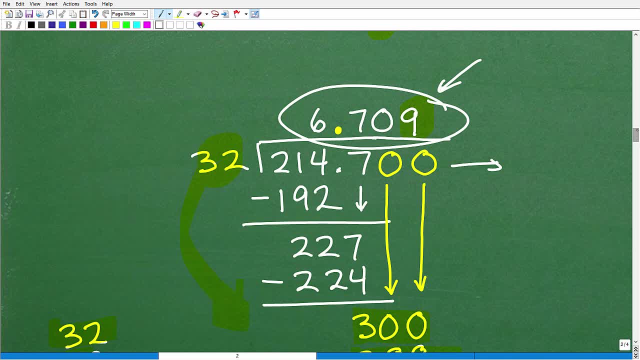 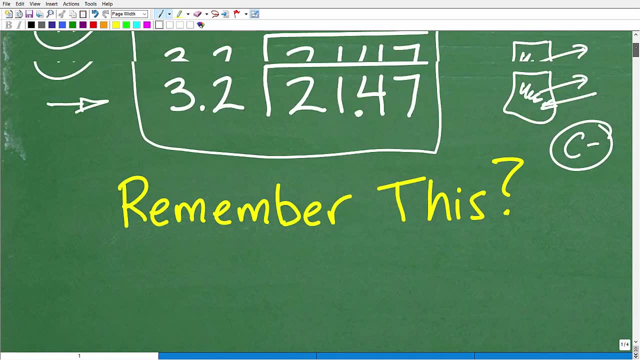 we can just increase its accuracy, But this is a basic example of dividing decimals And you know, if you forgot this, don't worry about it. You know most people have forgot this, but it's like riding a bike, You know. it's one of these things that maybe you have. 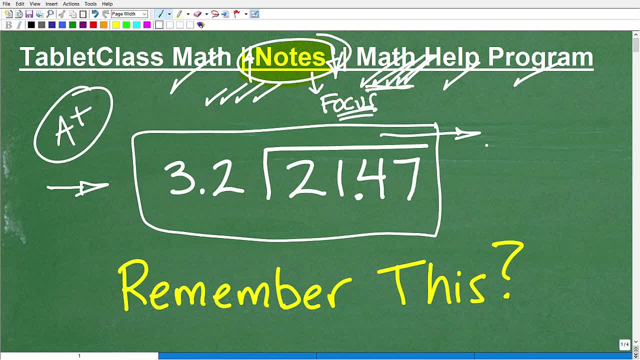 done in 20,, 30,, 40 years, But you're like, you know, after doing a few problems like this, you'll remember how good it felt to be in elementary school when you used to get a lot of happy faces and stars And a teacher would, just like you know, shower you with all kinds. 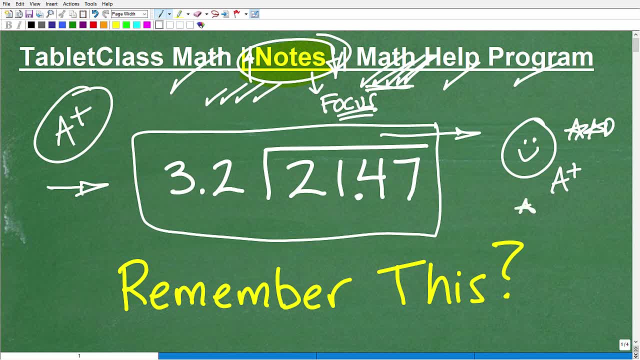 of rewards. Little Billy, you're so great at math, Here here's a couple extra bonus stars. And you were just so proud. And then something happened when you went to high school, right For the most of us we were like, yeah, I don't like school, or. 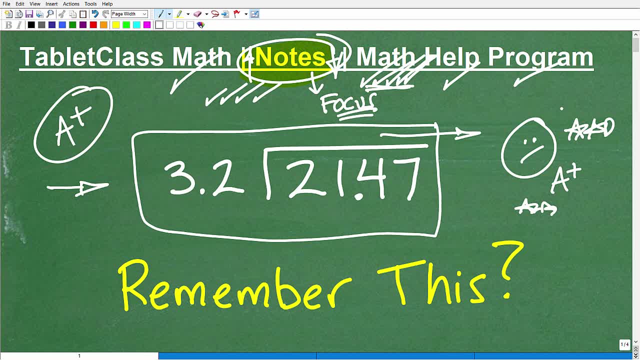 you know I'm speaking for myself. You know I'm too cool for math. Anyways, listen, elementary school. hopefully most of us have some good memories there, But if you remember how to do this, that's pretty impressive. OK, of course, if you are recently out of school, then that's like.